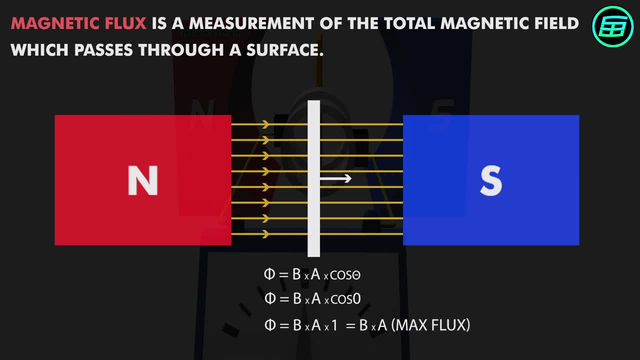 the flux is zero, there won't be. a current Formation of electric current depends on the change of flux, which can be calculated by this formula If the angle between the area vector and the magnetic field is zero. the rate of change of the flux is zero If the angle between the area vector and the magnetic field is zero. 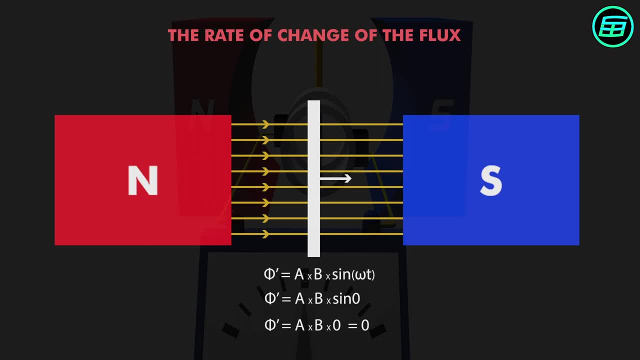 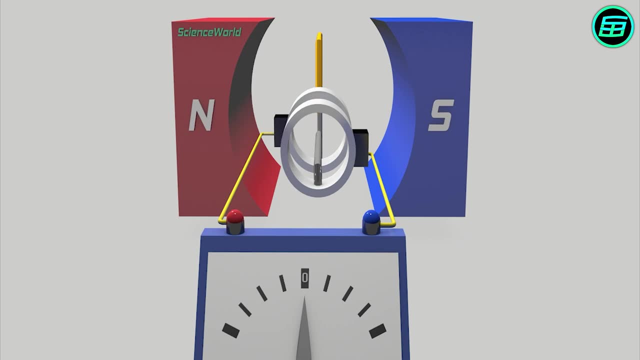 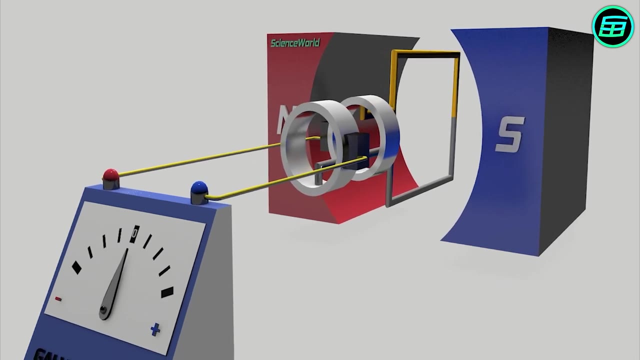 the rate of change of the flux is zero. The rate of change of the flux is zero When the armature is parallel to the magnets. the rate of change of flux is zero, so that no electricity is generated. But as the armature rotates, the magnetic flux starts to change. 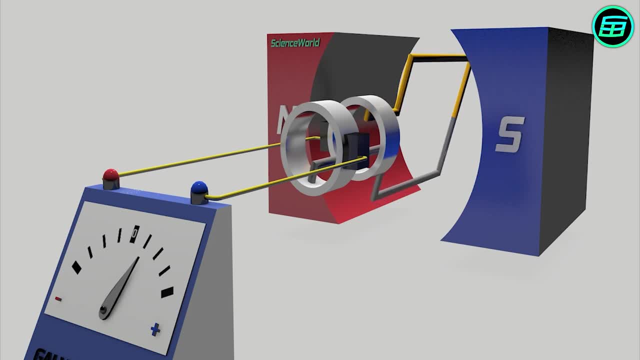 electrons in the armature start to flow and an electric current is formed. After a quarter of a cycle, the change of the magnetic flux reaches a maximum, and so the current reaches a maximum too, As the armature continues to rotate the change. 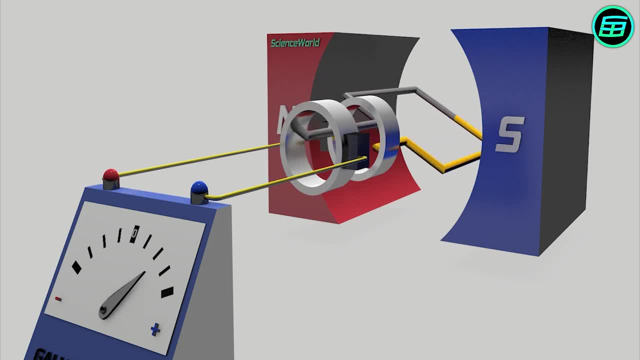 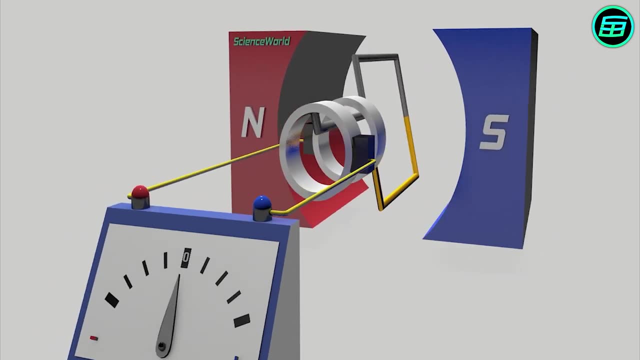 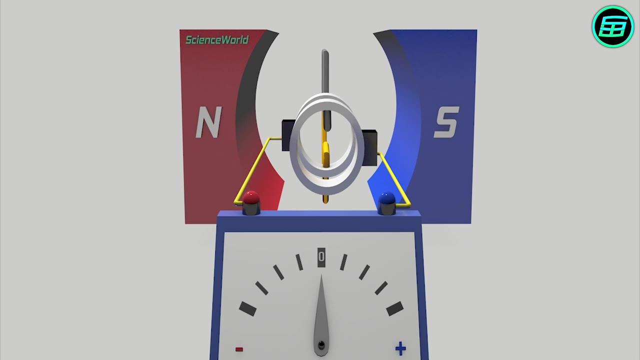 of the magnetic flux gradually decreases and consequently the current decreases as well When the yellow armature part reaches the bottom. the armature is parallel to the magnets and because the change of magnetic flux is zero at this point, the current is zero as. 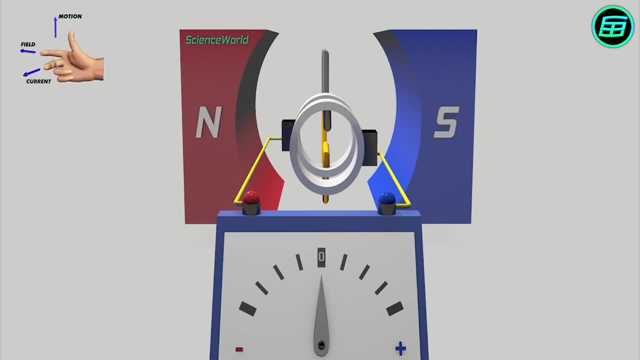 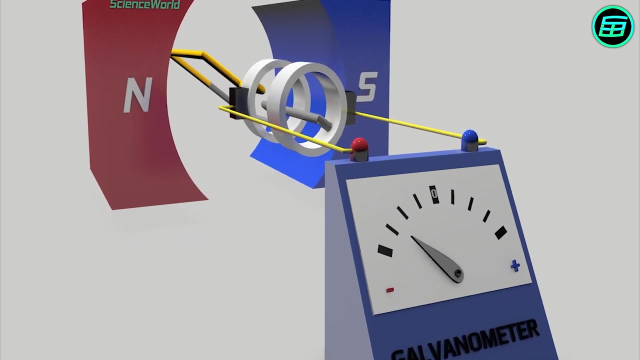 well Up to this stage. according to Fleming's right-hand rule, the current's direction is inward. As the armature keeps rotating, the magnetic flux starts to change again and reaches its maximum when the yellow armature part approaches the magnet. As the armature rotates further, the change of the magnetic flux decreases until it becomes. 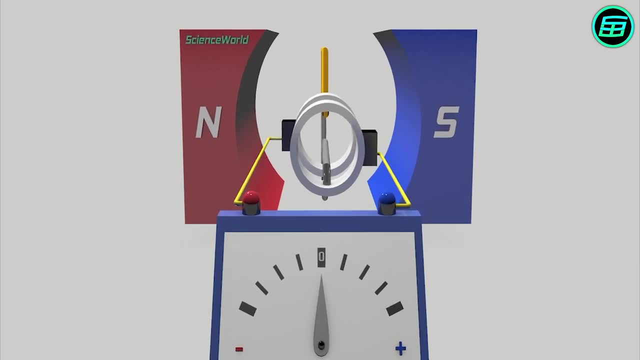 zero and the cycle is completed Between half and complete cycle. Fleming's right-hand rule indicates that the direction of the current, as shown here, is workable And by doing direction of current is outward. So every quarter cycle the electric current reaches. 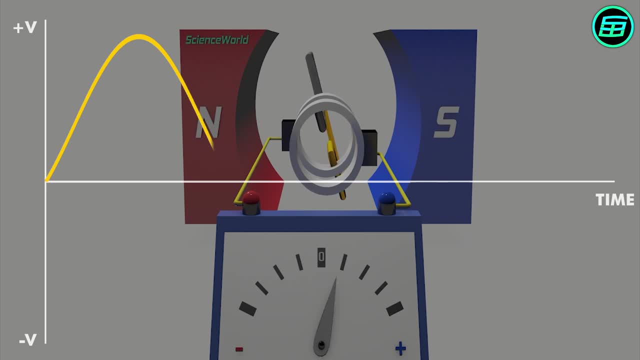 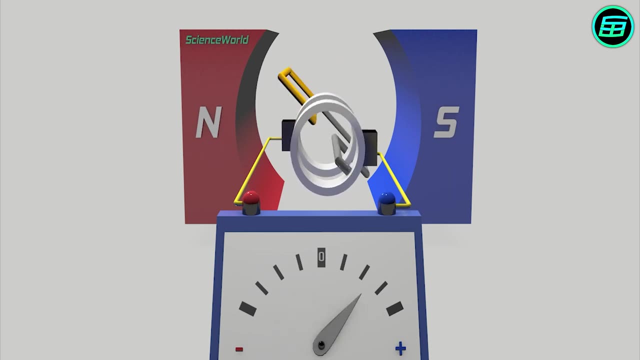 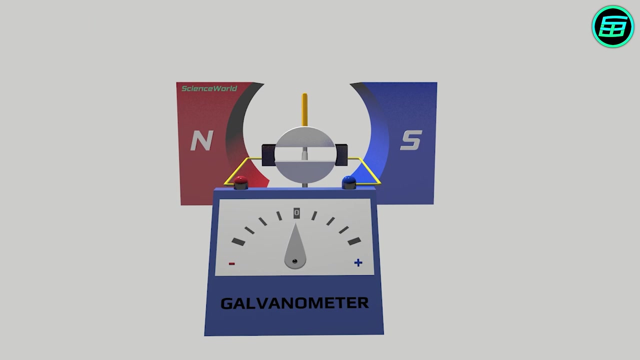 a maximum and every half cycle the current drops to zero. After every half cycle, the direction of the current changes. This change of the direction of the current is the biggest difference between alternating current and direct current. In direct current, in order to prevent changes of current direction,